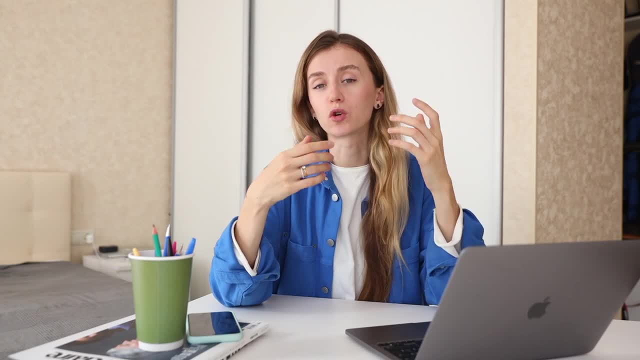 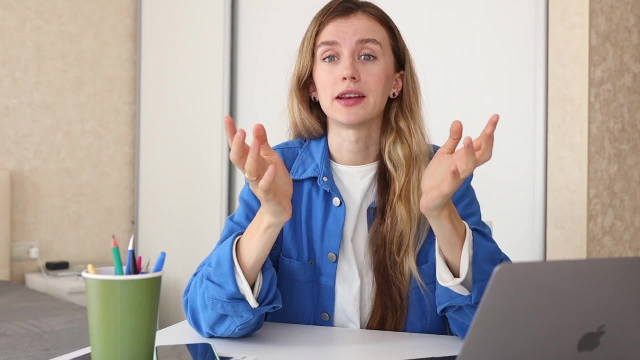 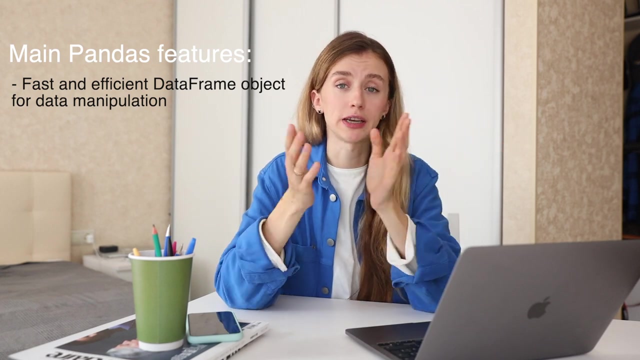 Plus, Pandas has so many in-built methods for grouping, combining, concatenating data and filtering, And it really has a wide variety of tools for analysis. Main features offered by Pandas are fast and efficient data frame object for data manipulation, pivoting and filtering of data sets. 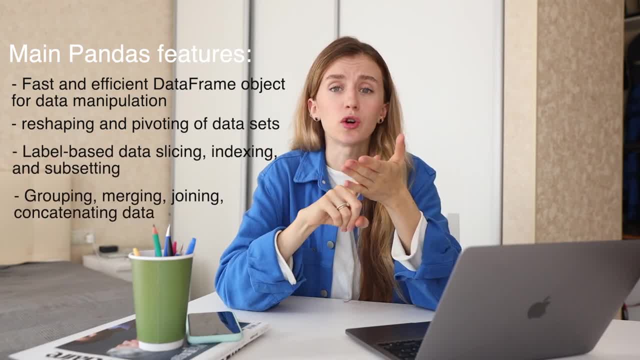 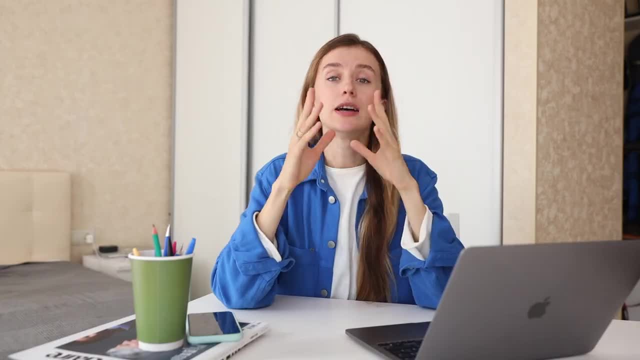 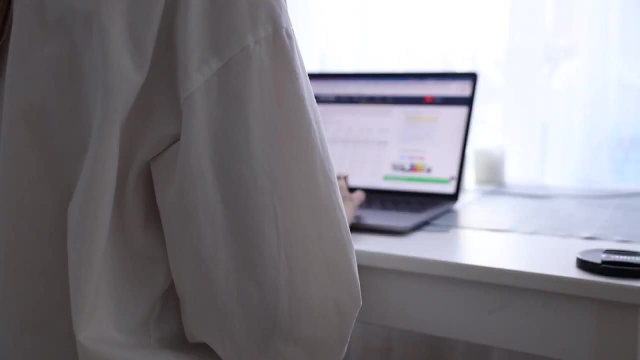 merging, combining, concatenating, joining data and- one more important thing- work with time series data So many. This library ensures high functionality and good amount of flexibility. Moreover, machine learning libraries also revolve around Pandas data frame as an input. 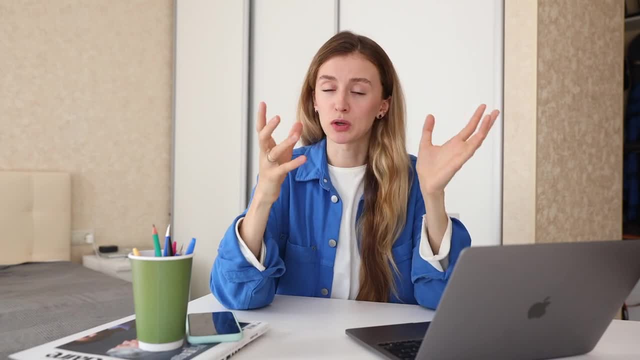 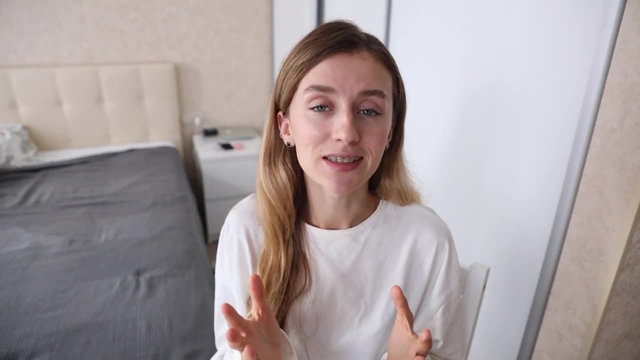 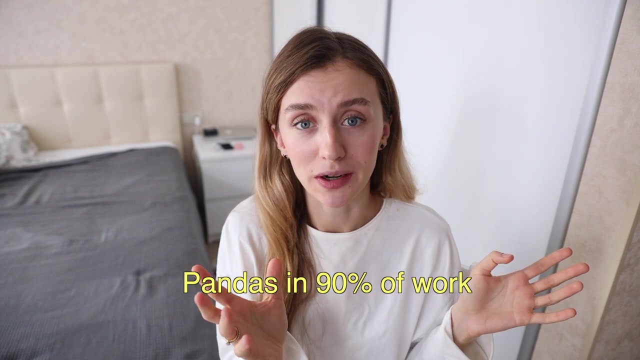 So if you need more information, so if you need best data analysis and manipulation tool, install Pandas. I asked my friends who work as data analysts what libraries do they use, and almost all of them answered that they use Pandas in 90% of their work. 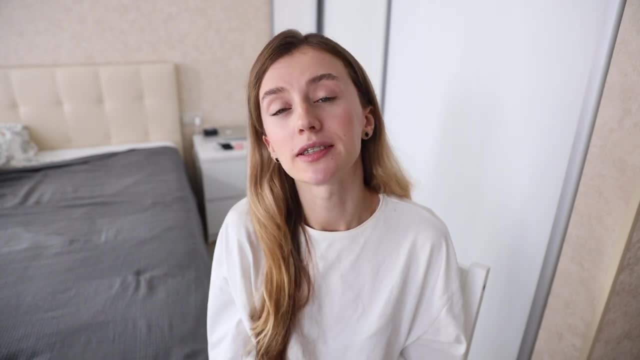 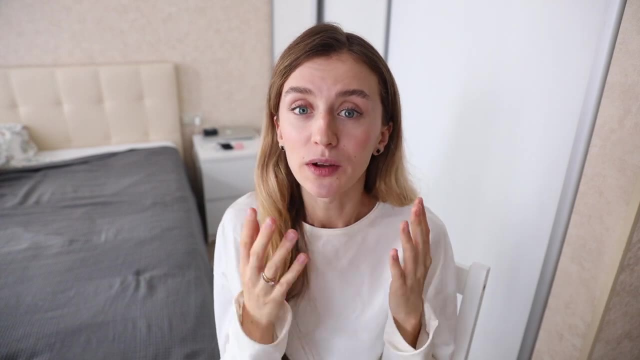 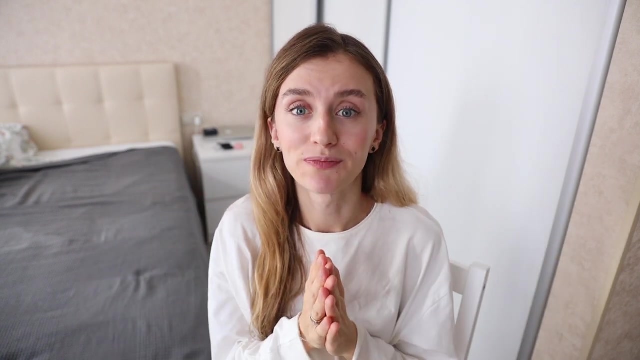 As for me, one of the part of my work is collecting data from open sources. That's why I also use parser libraries. So if you're interested in this topic- I mean parser libraries- please write in the comments below. I'll do separate video. 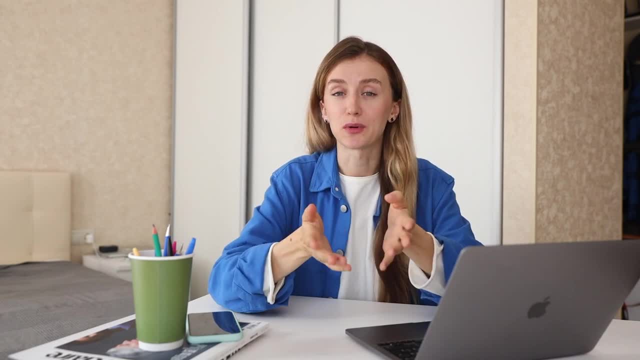 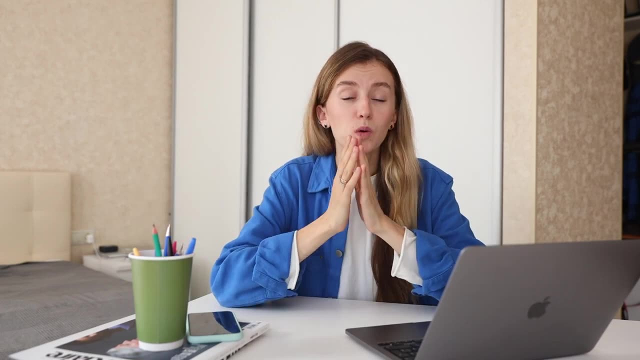 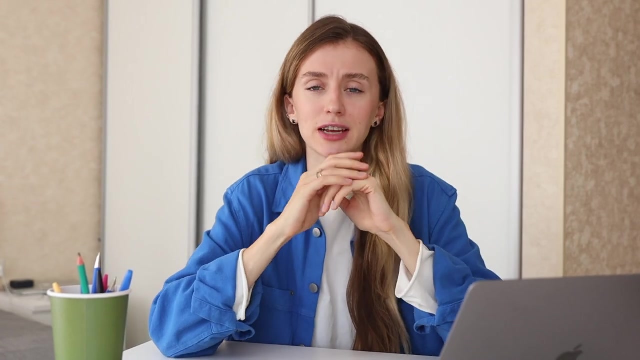 Next is NumPy. NumPy is mainly used for its support for n-dimensional arrays, And NumPy is easy to use and it makes complex mathematical calculations very simple. We can do any operations on NumPy arrays, for example subtractions and divisions, find, mean, median etc. 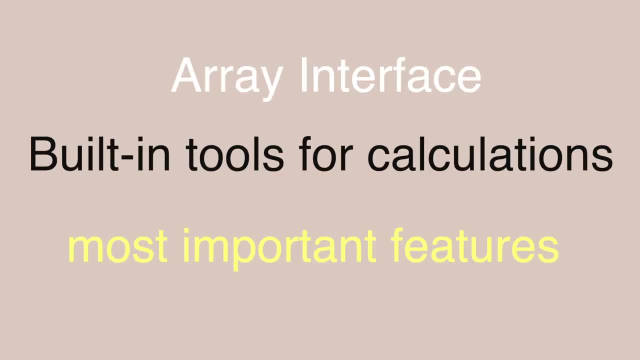 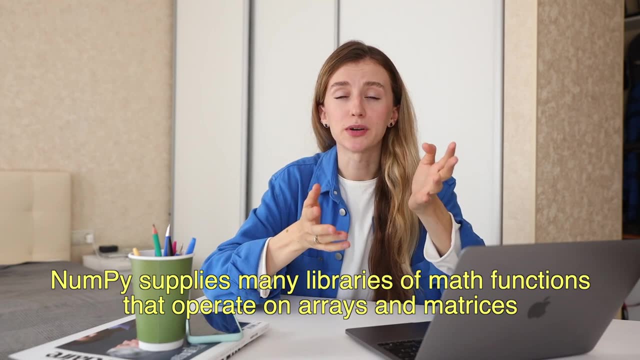 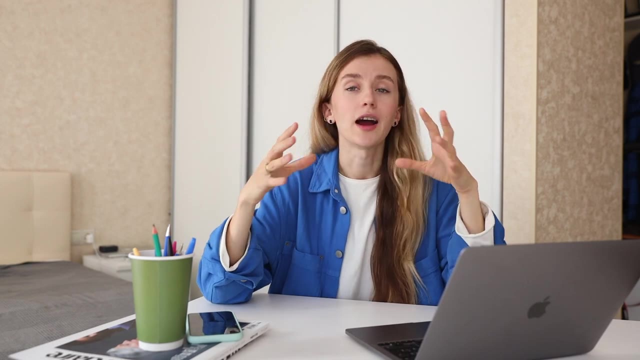 So array interface and built-in functions for mathematical calculations. mathematical calculations are the most important features of NumPy. I should say that NumPy supplies many libraries of high-level mathematical functions that operate on arrays and matrices, but still, if you need higher level of data analysis, 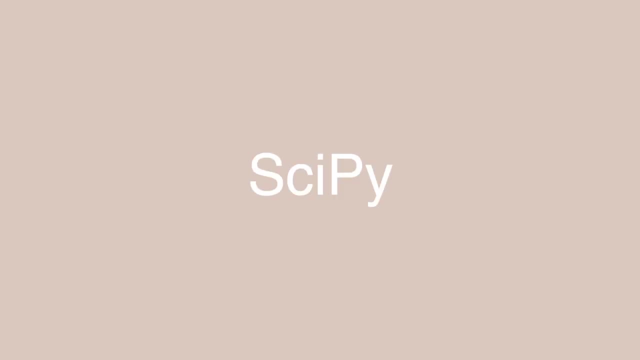 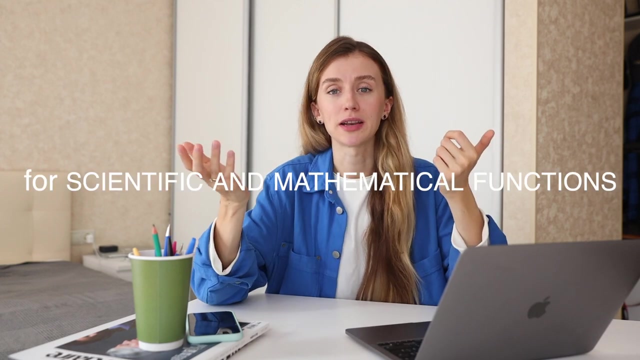 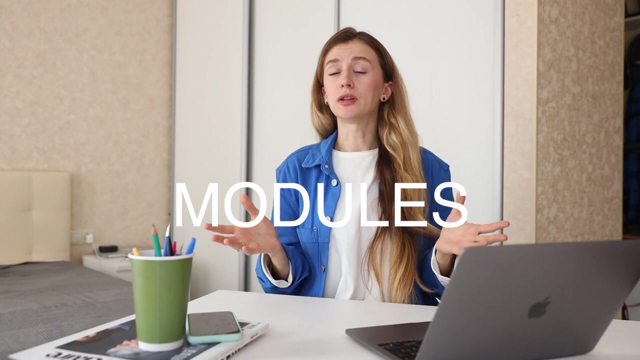 please use Pandas. Next library is SciPy. SciPy is a library that uses NumPy. It's mainly used for scientific and mathematical functions. It uses NumPy arrays as a basic data structure and it comes with modules for various commonly used tasks in data science and data analysis.